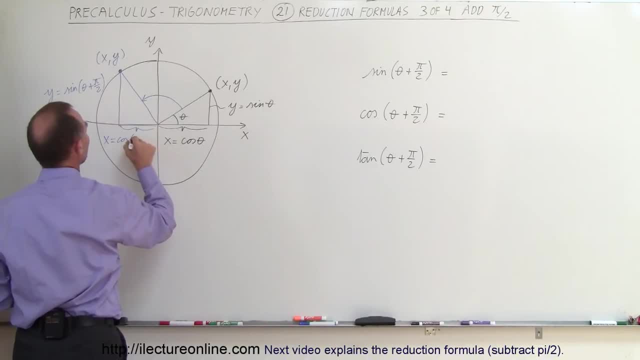 So the new x is equal to the cosine of theta plus pi over 2.. Now can we find a nice relationship? And the answer is yes. Notice that this is a right angle triangle. So is this, And actually those two triangles are exactly the same. 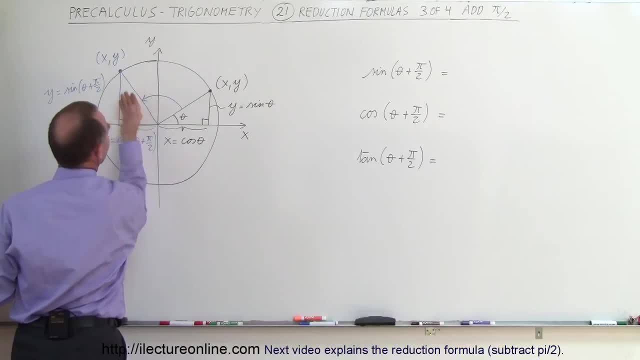 If you take this triangle right here and flip it over, make it look like that, then this right here becomes this value there And this right here becomes this value down there, Which means we can now relate the sine and the cosine to those angles. 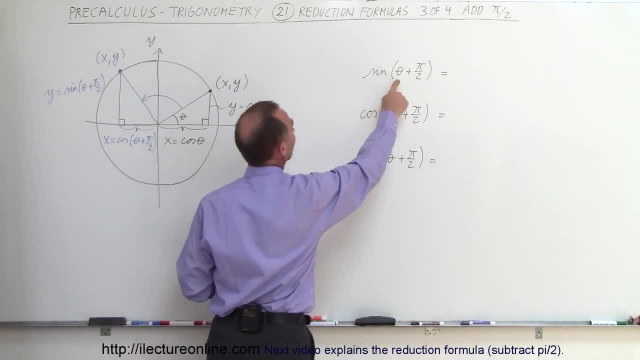 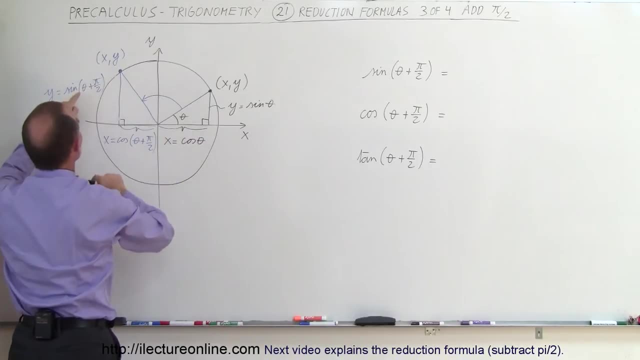 So let's try that. So, first of all, we have the sine of theta, pi over 2, which is this right here, And notice that this is equal to this value right there. That means that the sine of theta plus pi over 2 must equal to the cosine of theta. 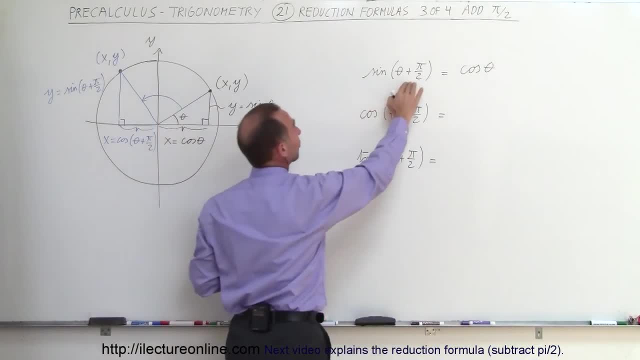 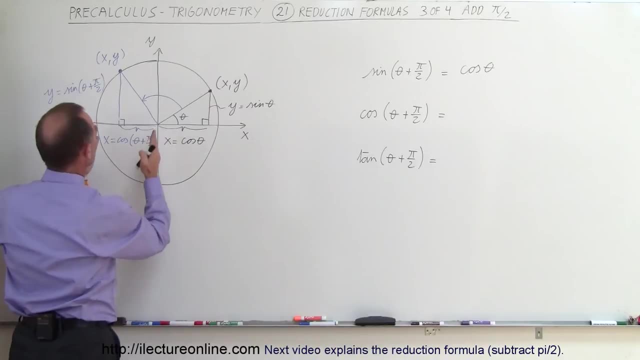 There And that's the relationship. So the sine of theta plus pi over 2 can be written as the cosine of theta. Alright, what about the cosine of pi plus theta over 2? That's this value right here. In size it's equal to this value right there, because those two triangles have to be equal. 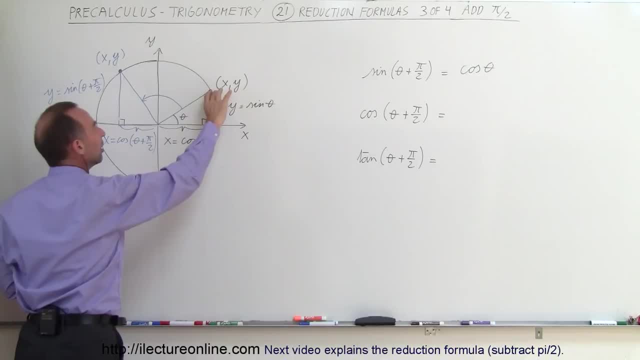 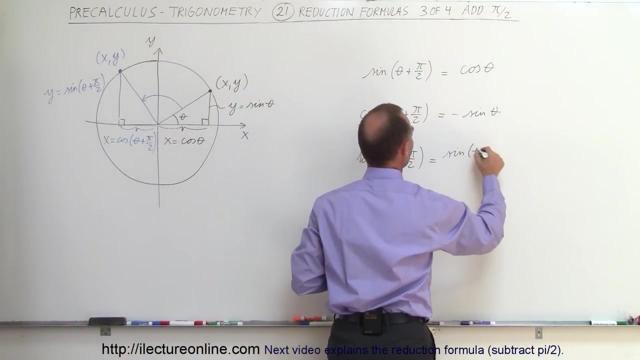 But it's on the negative side, so it becomes the negative value of this angle right there. So this becomes the negative of the sine of theta. And now for the tangent. since it's the, The sine, divided by the cosine, we can write this as the sine of theta plus pi over 2, divided by the cosine of theta plus pi over 2.. 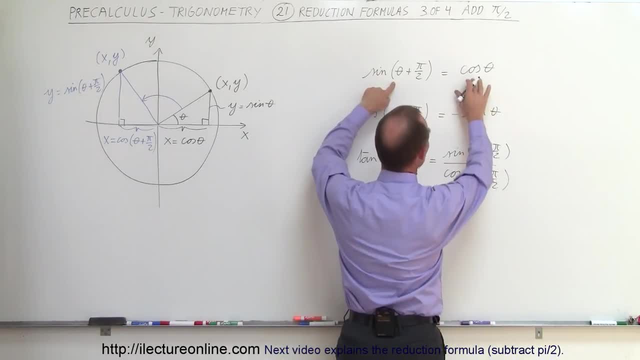 And notice that the sine of theta plus pi over 2 right here becomes the cosine of theta. so this is equal to the cosine of theta, And the cosine of theta plus pi over 2 becomes the minus, the sine of theta, And the cosine divided by the sine is the cotangent. 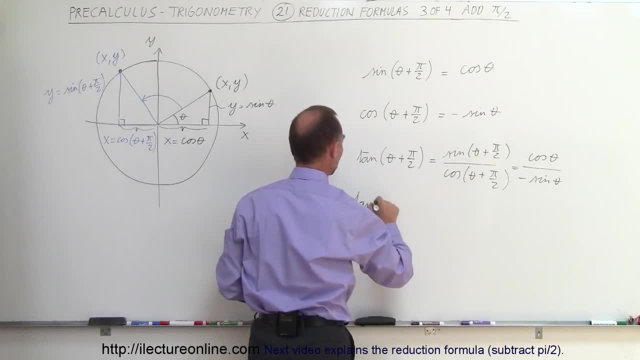 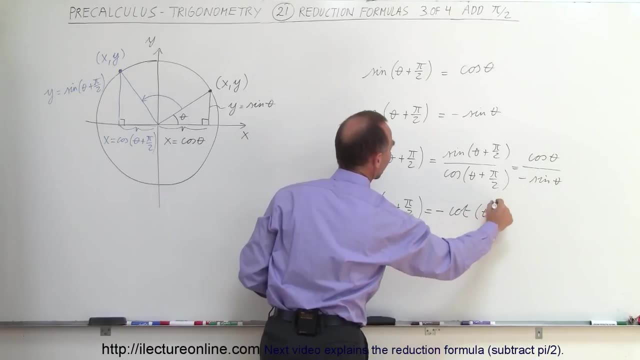 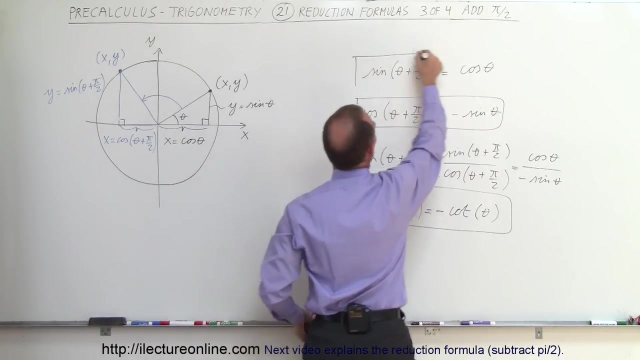 and we have the negative sign in front of that, which means that the tangent of theta plus pi over 2 becomes the negative cotangent of theta. And so these are the three reduction equations that are obtained when we add pi over 2 to the angle. 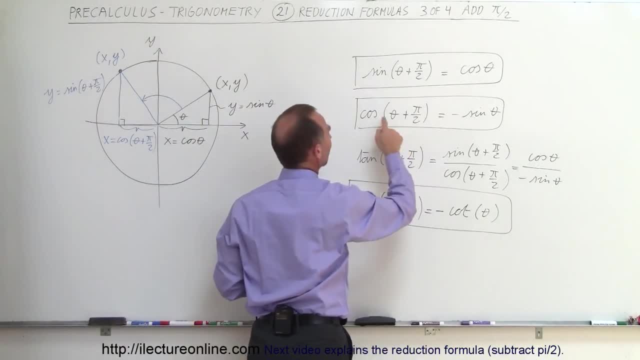 So, in the case of the sine, if we add pi over 2, it becomes a cosine. In the case of the cosine, when we add pi over 2, it becomes a negative sine. In the case of the tangent, when we add pi over 2,.